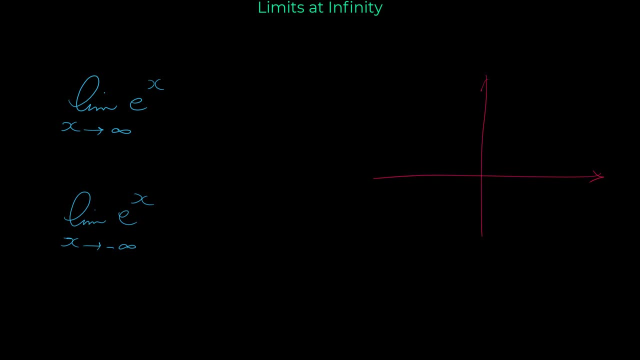 i highly recommend you memorize the graph of the exponential function e to the x. graph of e to the x is something like this. so this is the graph of the function. y equals e to the x, as you can see from the graph of megapix, when we go far to the right, when x approaches infinity being, 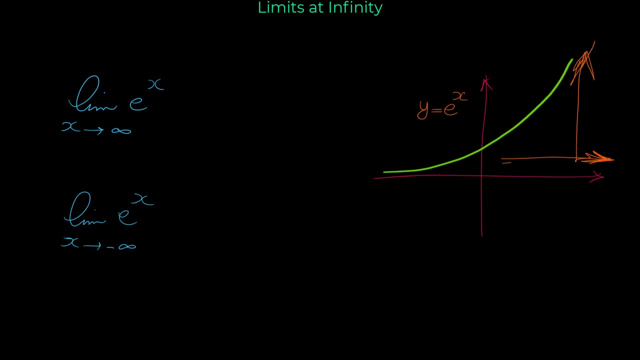 the y value of this function goes to infinity when we go far to the right, which means that x goes to infinity. e to the x, the y value of this function goes to infinity. so limit of e to the x when x approaches is infinity. so the answer of the first limit is infinity. 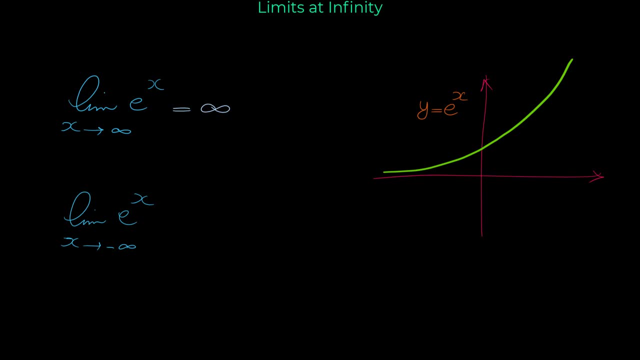 what is the limit of e to the x when x approaches negative infinity? now we have to look this way: what happens to this graph of e to the x if we go far to the left? as you can see here, when we go to the left, the graph of e to the x goes this way and it approaches: 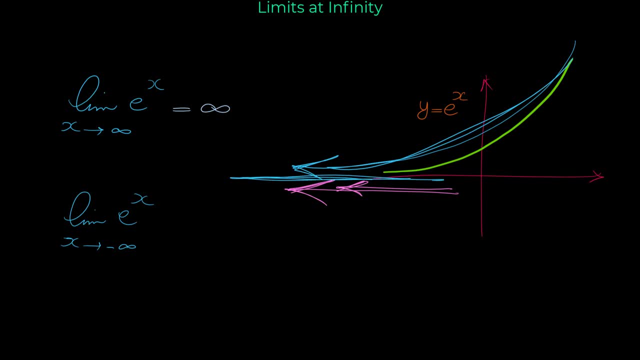 the x-axis. the distance between the graph of e to the x and the x-axis gradually decreases. so we can conclude that the limit of e to the x when x approaches negative infinity is zero. so the second limit is zero. and again, why this limit is zero? because attention to the 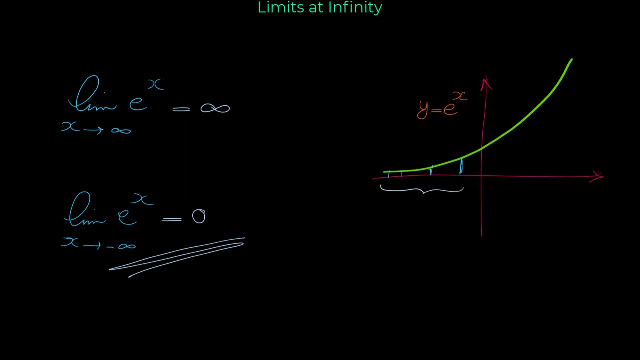 distance between graph of e to the x and the x-axis. this distance here gradually decreases when we go far to the left. this distance is almost zero. so the limit is zero. attention, this distance is never zero. but we can say that the limit of that is zero limit. 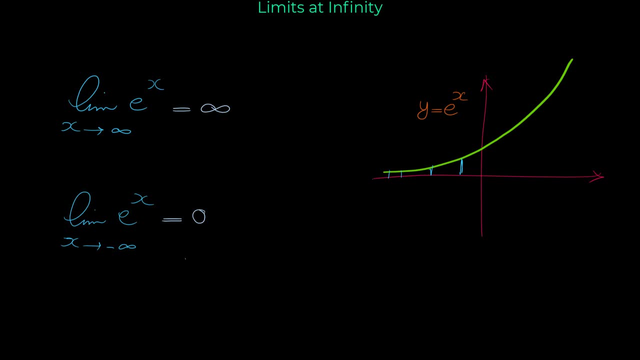 of e to the x. when x approaches negative, infinity is zero, and you can always remember these two limits, simply if you remember graph of e to the x. so, instead of memorizing these limits, it's better to always have graph of e to the x in your head and 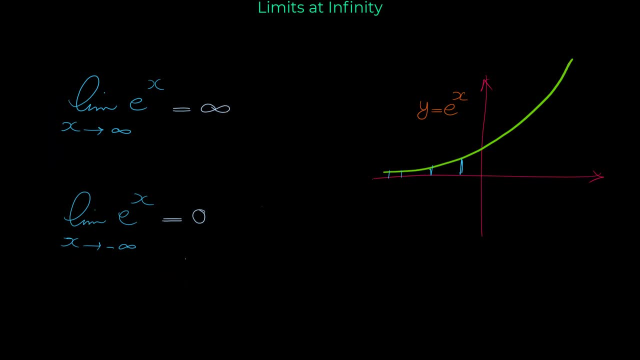 memorize it and then you can answer different questions and attention. not only graph of e to the x is like this. graph of many exponential functions are like this. in general, we can say that this is graph of any exponential function, like 2 to the x, 5 to the x, 10 to the x. but this is important, that the base 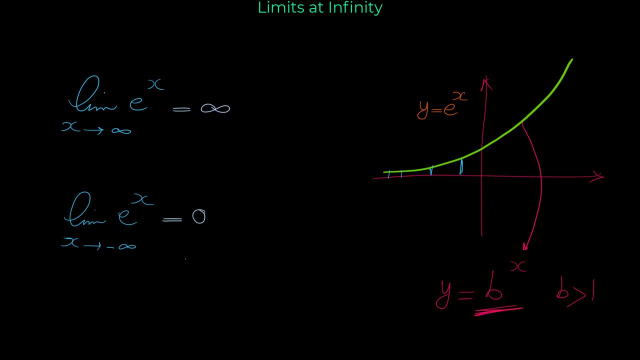 of your exponential function should be greater than 1. so as long as the base of the exponential function is any number greater than 1, like 2, 5, 10 and so on, the graph is the same, and so we have similar rules for them. but if b is not greater than 1, is less than 1, is between 0 and 1, it would. 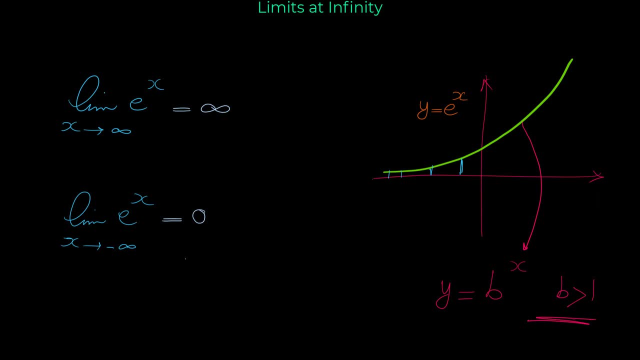 be different, the graph of b to the x. but mostly when we have exponential functions, the base of them is greater than 1, so we can use this graph for them. now look at these questions: what is limit of, let's say, 3 to the x when x approaches negative infinity? 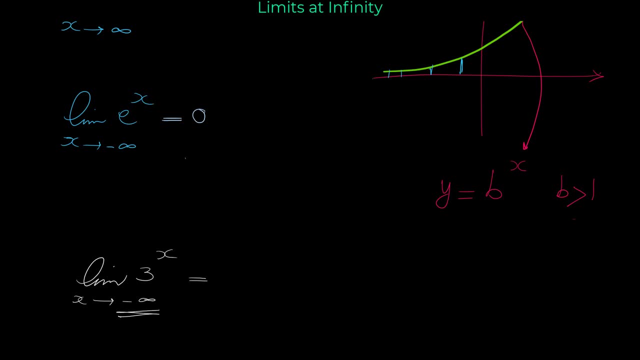 because x approaches negative infinity and the graph of 3 to the x is similar to e to the x. so what is this limit? because x goes to negative infinity, the еч ال Selbst nastıozat is 0. what is limit of 5 to the power of 2x when x approaches infinity? when x 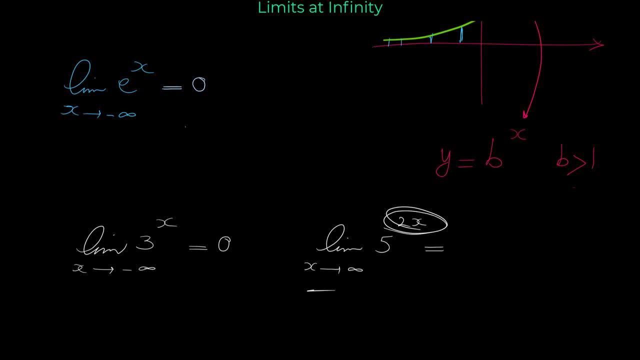 approaches infinity. 2x goes to infinity, and so basically we have this case. the base is 5 is greater than 1, and so the graph is similar to e to the x limit is also infinity, so this limit equals infinity. now look at this question: what? 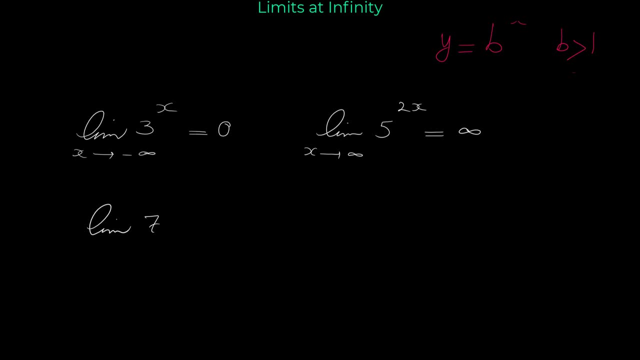 is limit of 7 to the power of x to the 2 plus x when x goes to infinity again, because x goes to infinity, infinity, this power is infinity and 7 to the infinity is infinity. so only you need to remember this graph and you can answer all of. 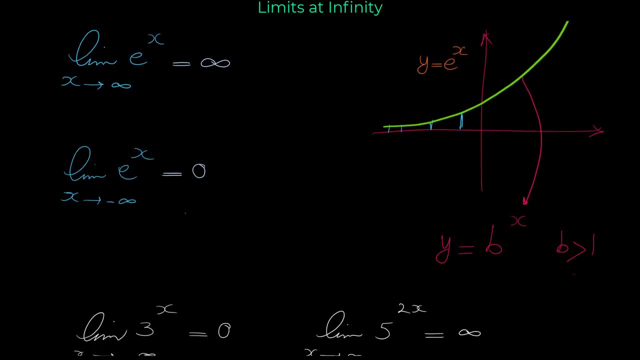 this question. when the x power is infinity, the limit is infinity. when the power is negative infinity, the limit of that exponential function is zero. now let's do some harder examples. we want to find the limit of e to the power of x, plus e to the power of negative x. 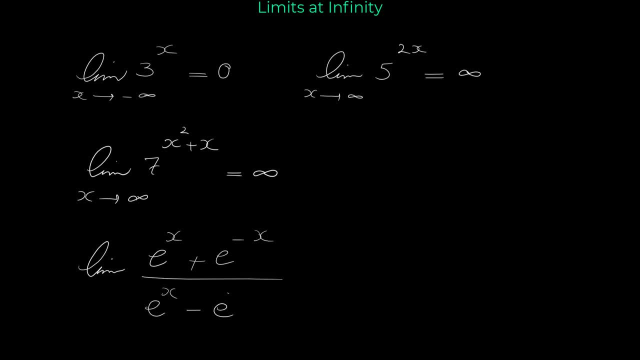 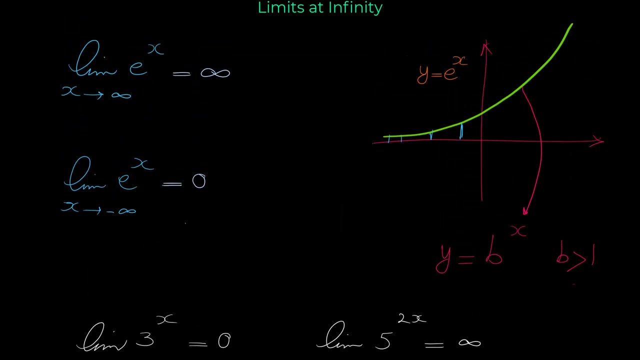 all over: e to the x minus e to the negative x, as x goes to infinity. when x approaches infinity, we know that. remember from here, limit of e to the x is infinity and limit of e to the x approaches negative if the exponent here it goes to negative infinity, the limit of that is zero. 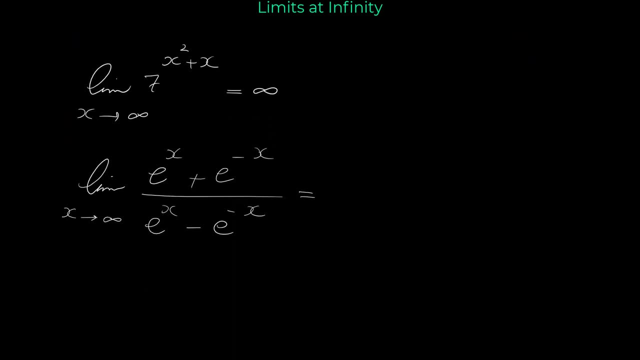 by considering these things. look at here: when x approaches infinity, the power here is infinity, so this goes to infinity. but when x approaches infinity, negative x approaches negative infinity, so basically this approaches zero. so between these two term in numerator, this term is the dominant term and this term approaches zero, so we can ignore it. 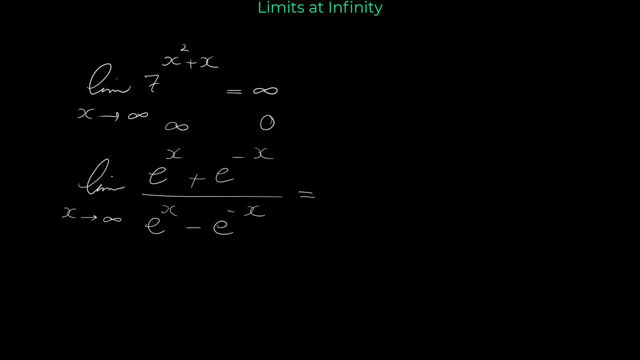 and similar thing we have in denominator between e to the x and e to the negative x. in denominator e to the x is the dominant term because it goes to infinity, but e to the negative x approaches zero. but if you do this, it in this way to say that we keep e to the x in numerator and e to the x from denominator. 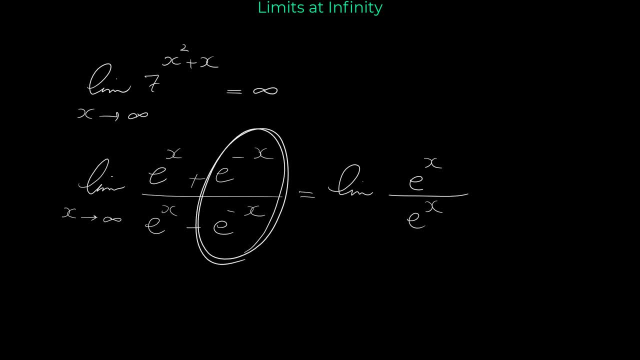 and we ignore these terms because the limit of this and limit of this is zero. if you do this limit in this way and from this you conclude that the limit is one, your answer is one, but your show work maybe is not enough. the limit of this expression is one, but how we can do this? 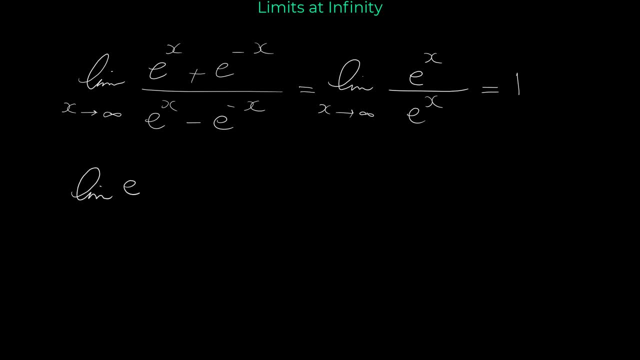 question in a better way. let me rewrite the question again. if you remember from limits of rational functions, when we have rational functions, rational functions are functions that in numerator we have polynomial, in denominator also we have volume. for finding limits of such functions. we divide numerator and denominator by highest degree of denominator. 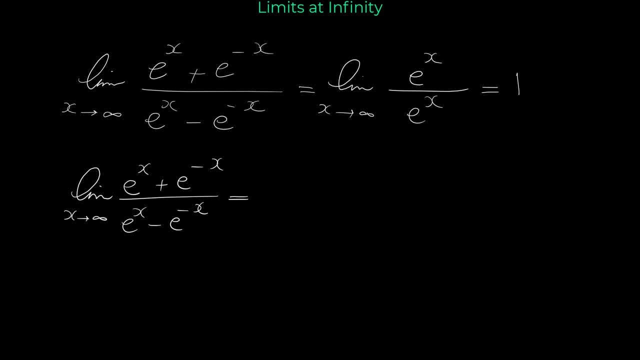 so, but here we don't have polynomials. but we can use same idea to find these limits here. look at the denominator and try to find between the two terms, that is in the denominator, which one is the dominant term. we can say the highest degree, because here we don't have polynomials. but you can think it this way, between this term and the 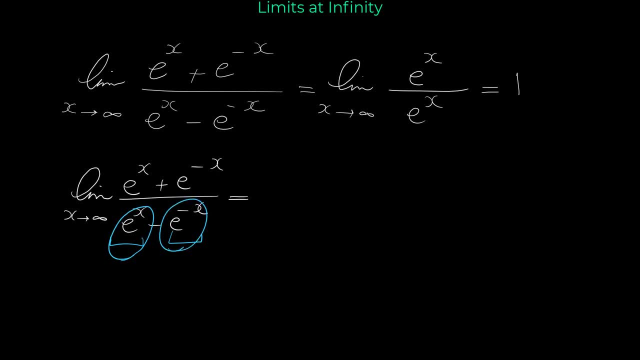 same this and which one is significant. or, if you want to compare it with polynomials, which one is the one with highest degree. if you remember, when x approaches infinity, this is infinity, this is zero. so this term is obviously the dominant term or significant term in the denominator. so, for finding 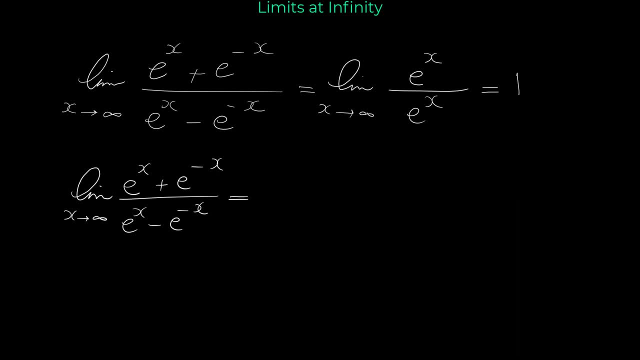 this limit. we are going to divide every time in the way and everything denominator by highest degree numerator. we are going to divide every term in numerator and every term in denominator by highest degree because of this limit that mean that we have jeito degree by the term that has the highest degree in denominator, which is e to the 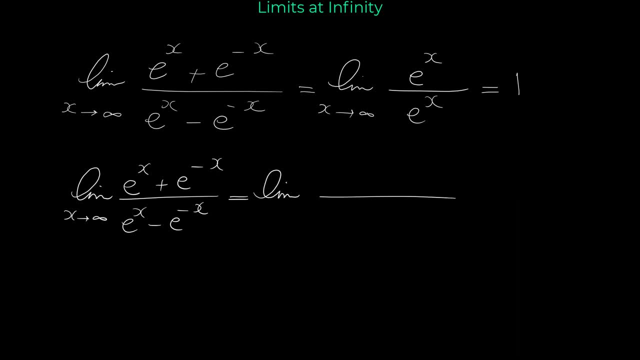 x. so we divide everything by e to the x, so e to the x over e to the x, e to the negative, x over e to the x. and same thing in denominator, and x approaches infinity. now by doing this we have limit of one plus e to the negative, 2x in a. 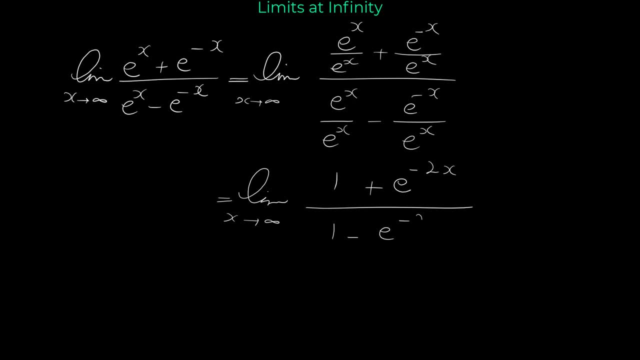 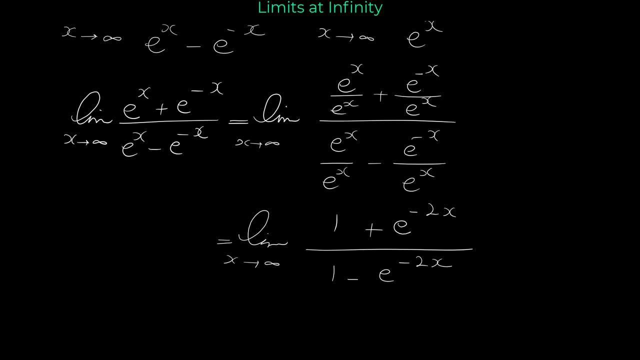 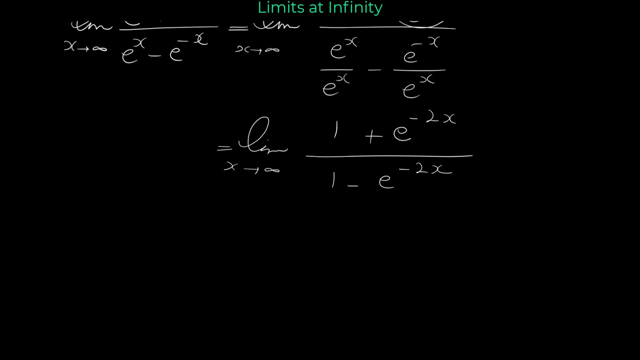 moment. I will explain you why. this becomes e to the negative 2x, e to the x over e to the x is 1, e to x over e to x is 1 and e to the negative. x over e to the x is e to the negative 2x. why? because attention, we have e to the 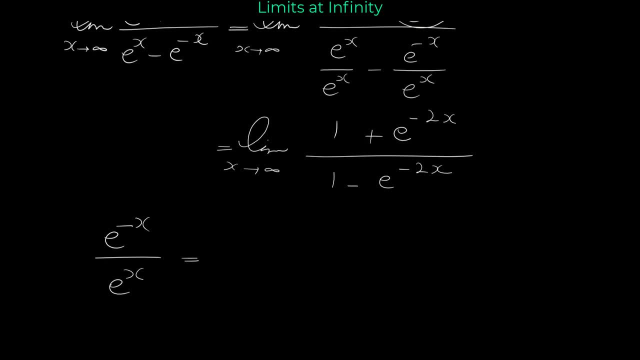 negative x over e to the x. when we have division between power expression we can write one of the bases and subtract the power. so this equals to e to the negative x minus x and this equals e to the negative 2x. now attention to the numerator and denominator. in numerator we have 1 plus e to the negative 2x, the. 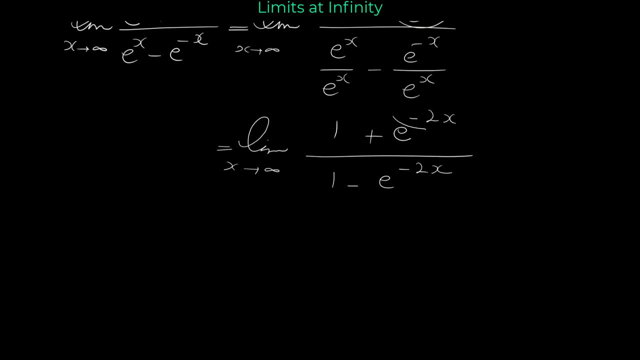 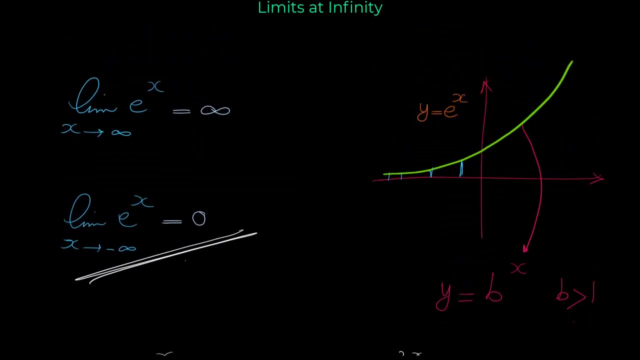 power of this exponential expression here, when x approaches infinity, the power here goes to negative infinity because of this negative here. and so we have basically this case: limit of e to the x when x approaches negative infinity is zero. when the exponent, the power of exponential function, goes to. 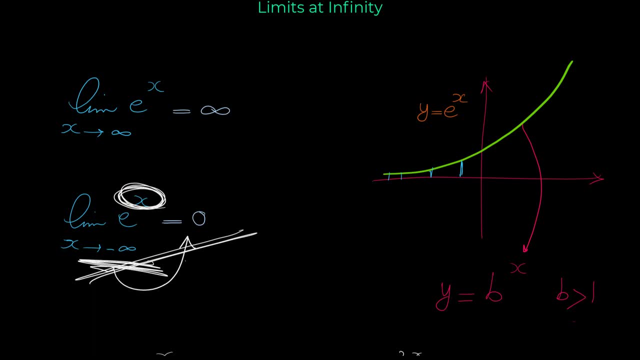 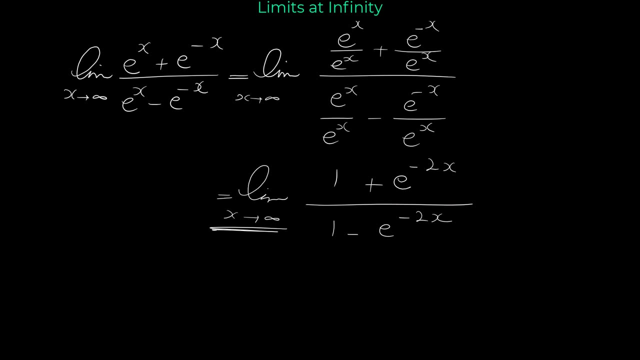 negative infinity. the limit of that exponential function is zero. so here the limit of e to the negative 2x is zero, and also in the denominator limit of e to the negative 2x is zero. so this equals to 1 plus 0 over 1 minus 0. 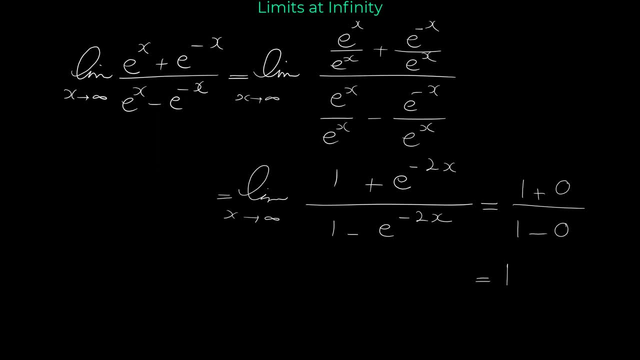 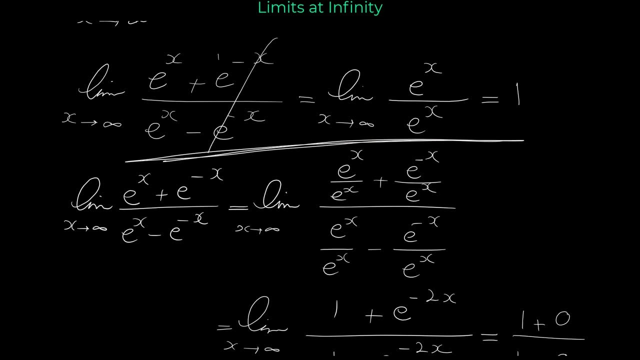 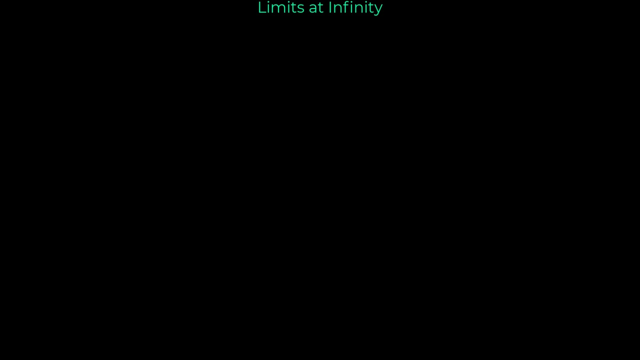 and so the limit equals 1, but of course you can use the other method which I showed you here, to ignore these terms and just keep the meaning of the definition, the real term. okay, so the next half step is keep the meaning of the definition, because we have하는 the Koran version, and make sure 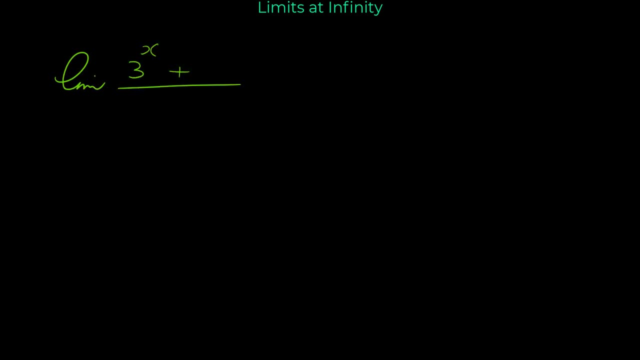 that what is written also is written in the clear Median. so all right, so here's our limit. the question is So: what is the limit of x plus 0 to the power of infinity? does it mean that we are going to give to the sum up for? 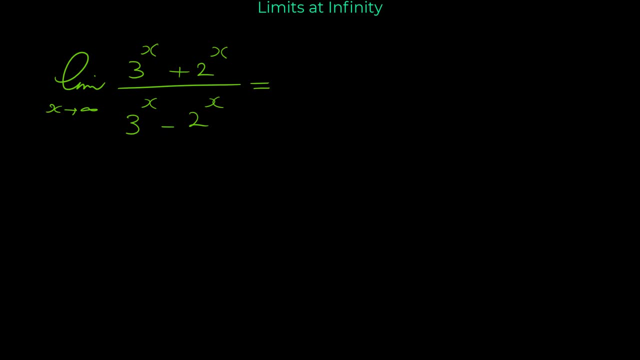 every time in the top and every time in the bottom, by their dominant, between 3 to the X and 2 to the X. which one is between these two term? which one is the dominant term? which one is the expression that grows faster? 3 to the X. 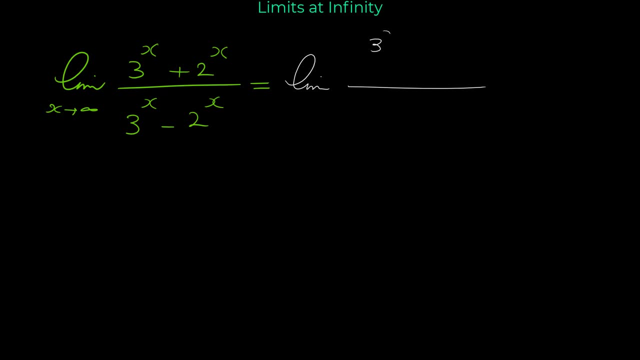 because the base is greater. so we are going to divide every term in numerator and every term in denominator by three to the X. then we have this: and X approaches in fact 3 to the X over. T to the X is 1, so we have 1 plus 2 to the X. 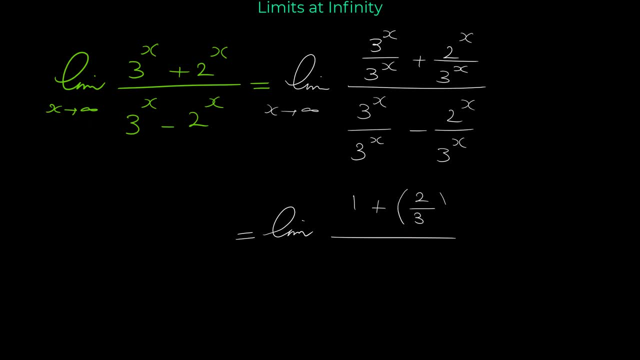 over T to the X can be written as one exponential function like this through Canon- Sorry for mistake: Solo. third to the x, and also we can do the same thing in the denominator and we can write as this: and, as you can see, sal happens to be the author name for the. 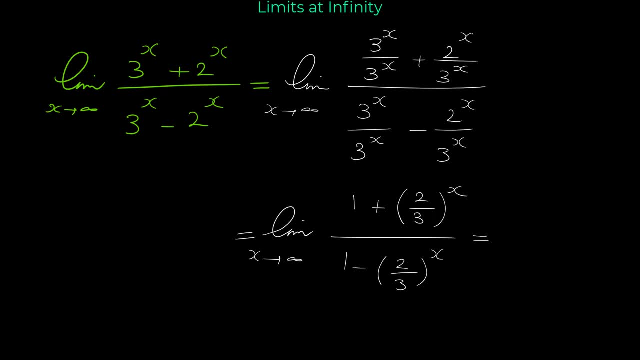 it this way now: x goes to infinity, so the exponent here goes to infinity. so maybe you think that you will have exponential function, that the exponent goes to infinity. so the limit of this is infinity. but attention here: the base of this exponential expression- here the base is 2 thirds- is less than 1. and when the base of exponential function is less than 1, if the 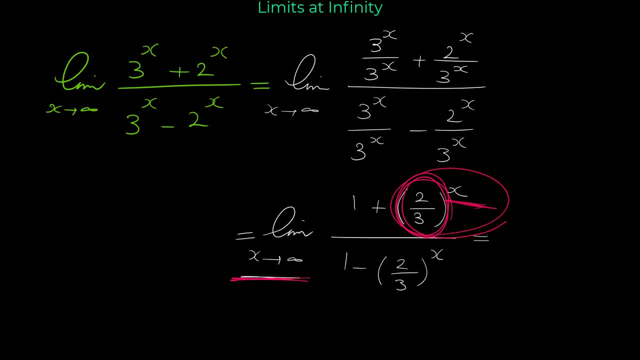 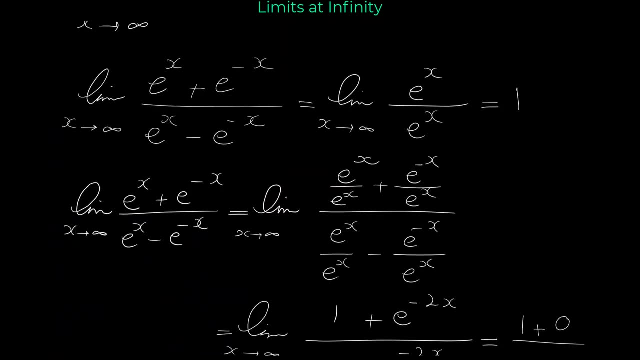 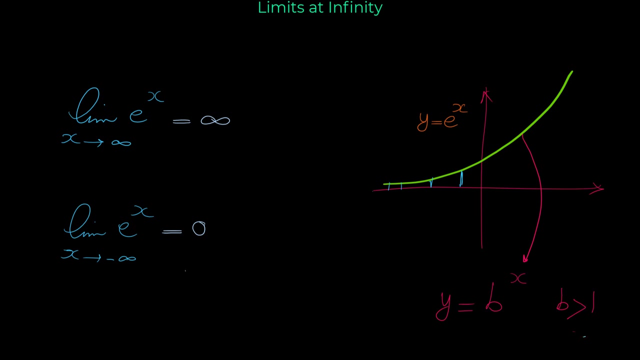 exponent goes to infinity. limit of that expression is 0, if you remember. graph of e to the x. for any exponential function is like this, but we had a condition here: if the base is greater than 1, the governing function would be 0. so, as you can see here with the exponential function, if you 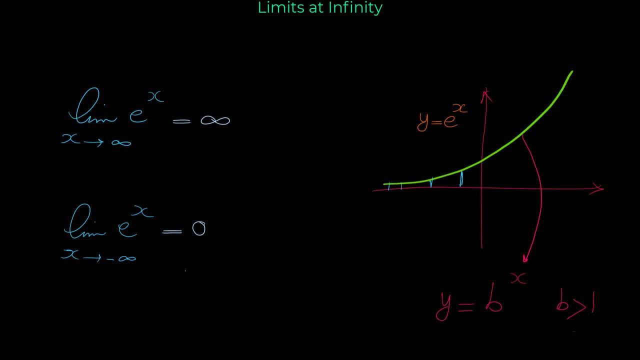 graph is like this: if the base of the exponential function, if the base of the exponential function B to the X is a number between 0 and 1, like one half 2 over 3 numbers between 0 and 1, the graph would be like this and, as you can see, if 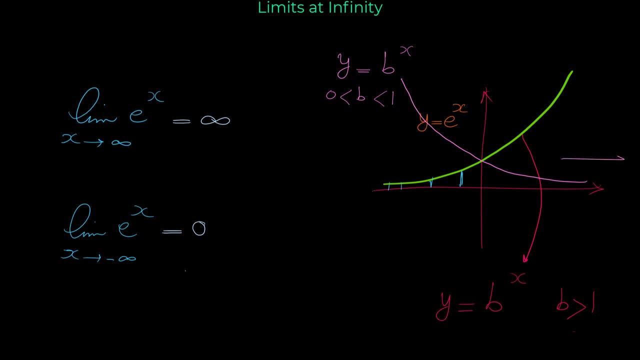 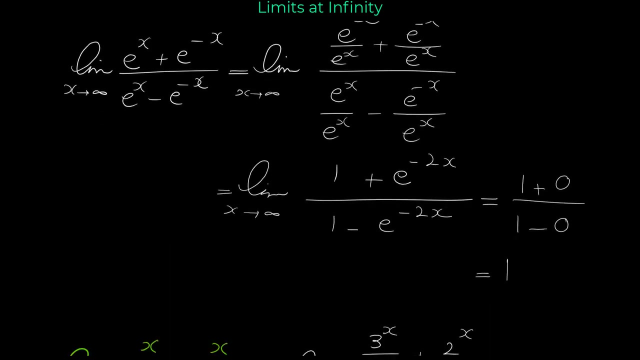 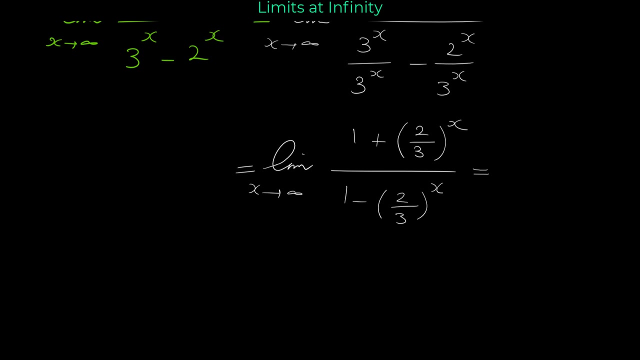 your attention to this new year. when we go far to the right, this function approaches 0 and in opposite, when we go far to the left, the get out of this function goes to infinity. so now, here in this limit, we have a number that is less than 1. when we traces to X, and X goes to infinity, the limit of that is 0. so we